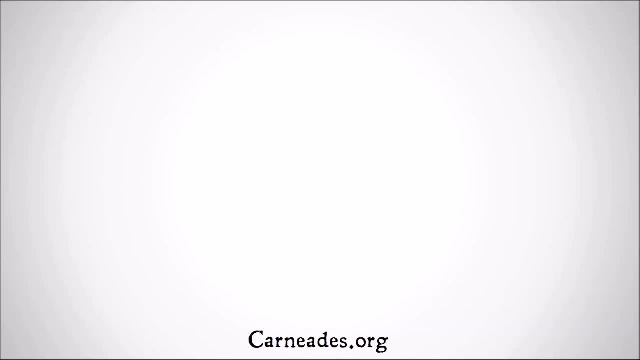 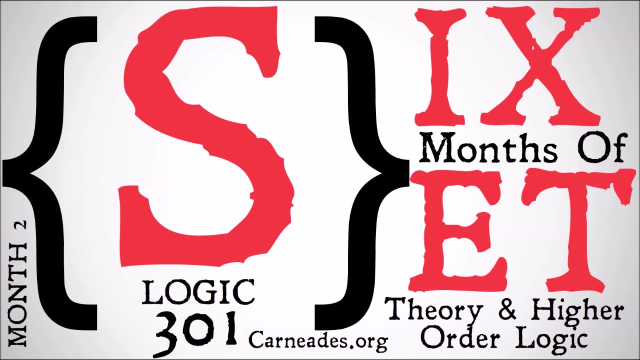 Welcome back to carnadiesorg. Today we're going to be continuing with our series six months of set theory and higher order logic, with a new video every single day for the whole month of October. This is month number two looking at operations and relations of sets. Today we are finally moving. 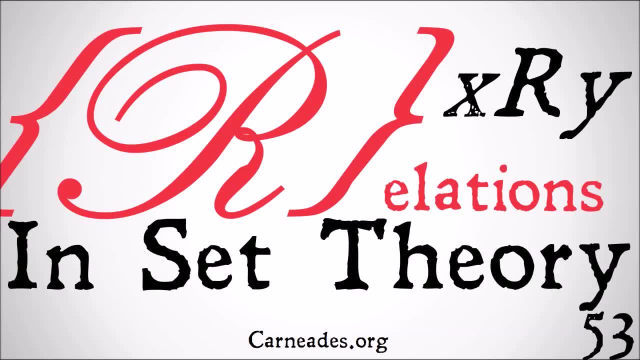 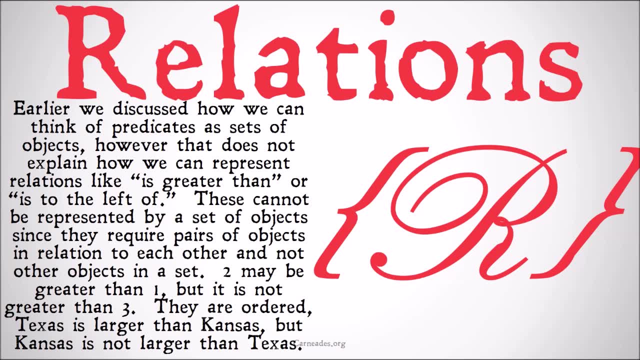 on from operations to relations in set theory. Now, earlier we discussed how we can think of predicates as sets of objects. However, that does not explain how we can represent relations like is greater than or is to the left of. is the father of is next to. These cannot be represented. 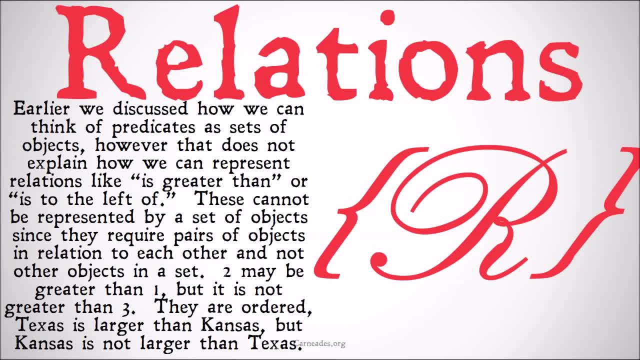 by a set of objects, since they require pairs of objects in relation to each other and not other objects in a set. Two may be greater than one, but it's not greater than three, So I can't just have a set of things That are greater than, because you need two objects paired together. They are ordered: Texas is larger. 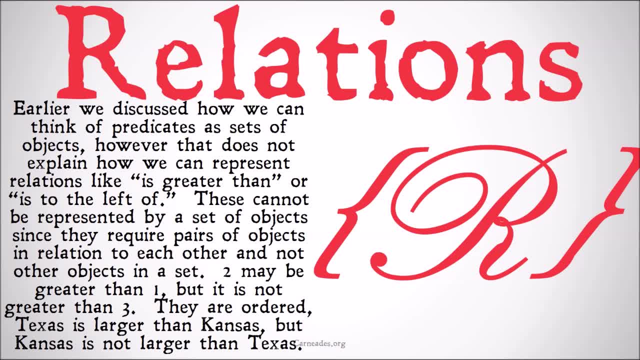 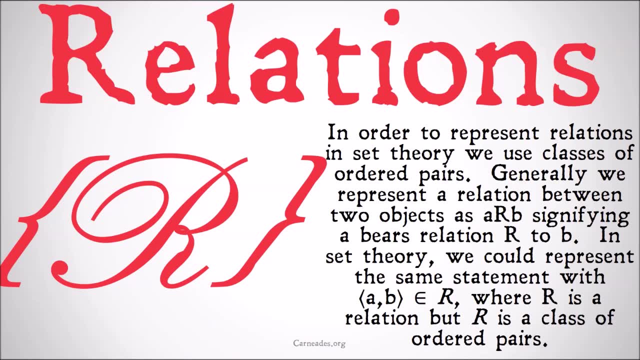 than Kansas, but Kansas is not larger than Texas. You can't necessarily switch them around, So relations are going to require a little bit different machinery to represent. Fortunately we have that. In order to represent relations, we're going to use classes of ordered pairs. 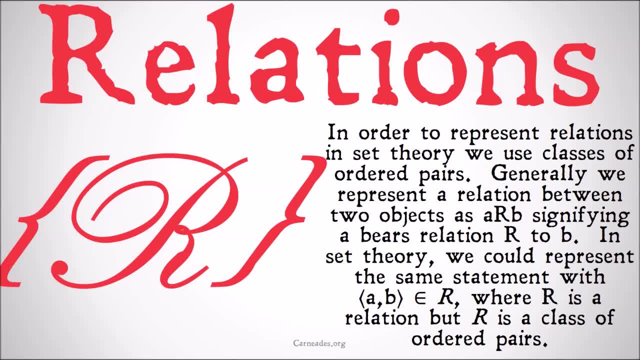 Generally we represent a relation between two objects, as a, r b, signifying a bears relation r to b. In set theory we could represent the same statement with the ordered pair a. b is a member of r where r is a relation. 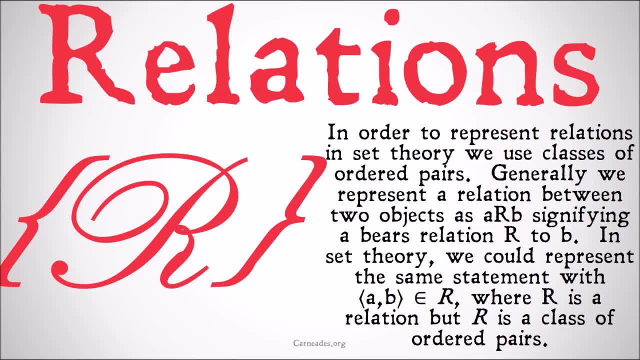 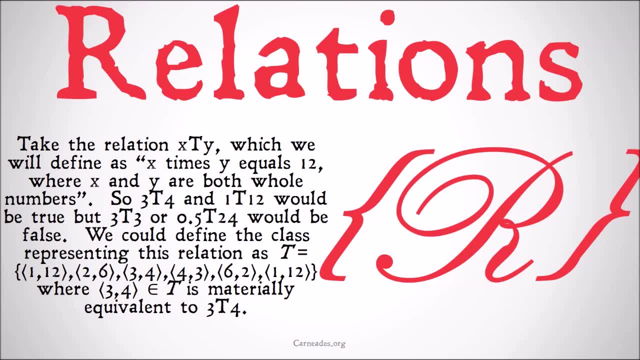 but r in italics is a class of ordered pairs. Take the relation x, t, y, which we'll define as a set of objects. x, Y equals 12. Where x and y are both whole numbers. So 3. T4 and 1. T12 would be true. 3 bears the 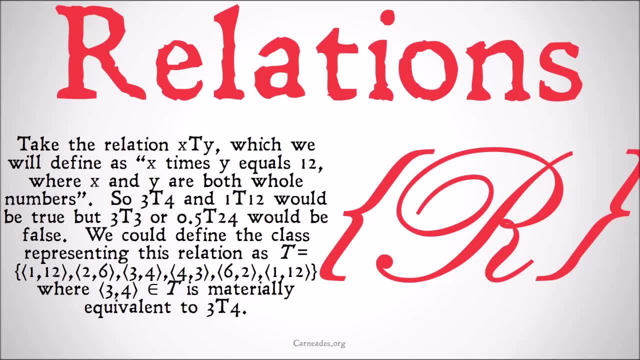 relation 3001.0 KB equals twelve to four and one bears the relation. 1 times twelve equals 12 to twelve, but 3�ные rrando 3t3 or point 0, 5 lesser leave 14122.000.0024. 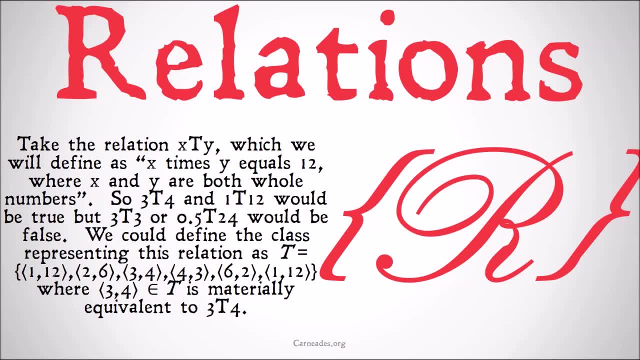 KB 24.2 would be false, 0.9103.1141.. одну Planner, 10 commandments, Since 3 and 4 equal To. let's go to the next section. pero it's 3 times 3 don't equal 12, and 0.5 isn't a whole number. 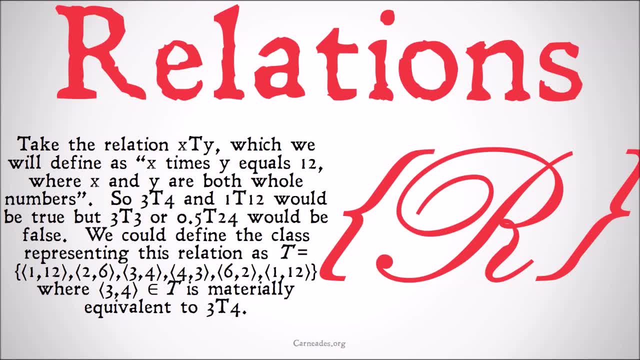 so it doesn't fit all of the criteria of the relation. We could define the class representing this relation as T is the class of the ordered pair 1, 12,. the ordered pair 2, 6, the ordered pair 3, 4, the ordered pair 4, 3,. 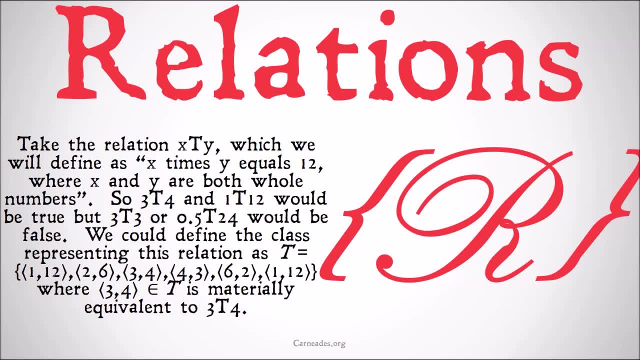 the ordered pair 6, 2, and the ordered pair 1, 12.. Note: we have to do both directions for all of those ordered pairs because they are explicitly ordered Where the ordered pair 3, 4 is a member of T. 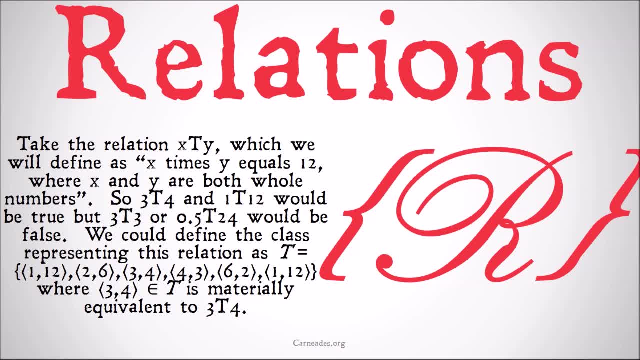 is materially equivalent to 3, T, 4, where T in italics represents the class and T, not in italics, represents the relation. Some authors may use them interchangeably and not distinguish between the class and relation, just basically defining the relation as the class. 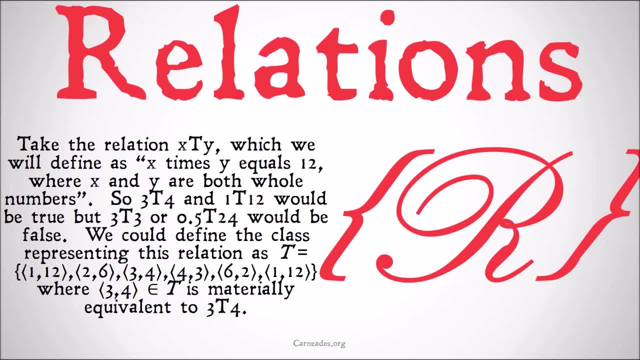 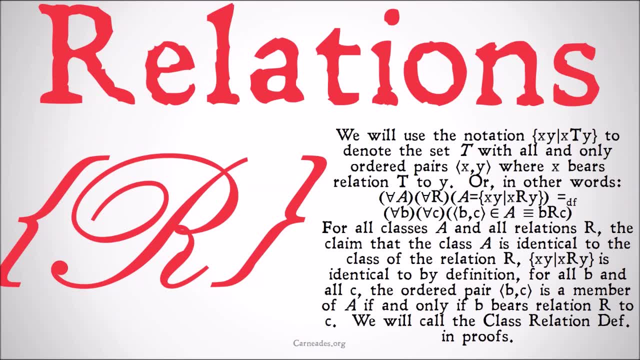 Here I'm going to be a little bit more specific, but only within the nuance of definition. I'm not doing italics or not. We're going to use the notation class of xy, bar xty, to denote the set T with all and only ordered pairs xy. 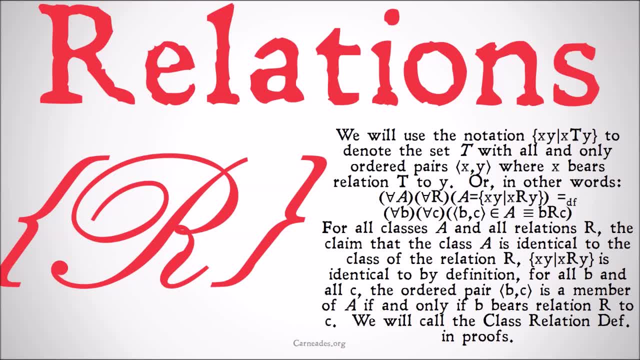 where x bears relation T to y, similar to the predication relation that we looked at earlier or the predication symbol that we looked at earlier, Or in other words, for all a and all r, a equals this class of the relation, r. 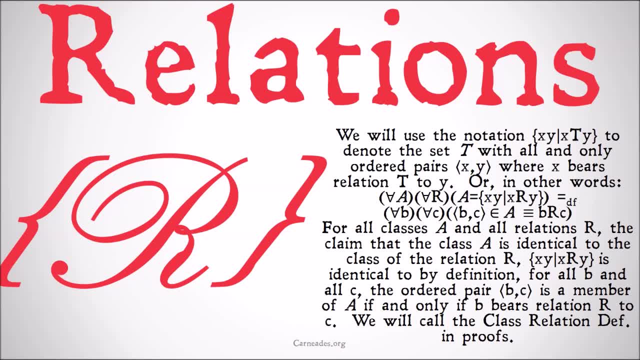 means by definition for all b and all c, where note that those b and c are not in italics. They are objects, They are things. They're not necessarily sets or classes. The ordered pair bc is a member of class. 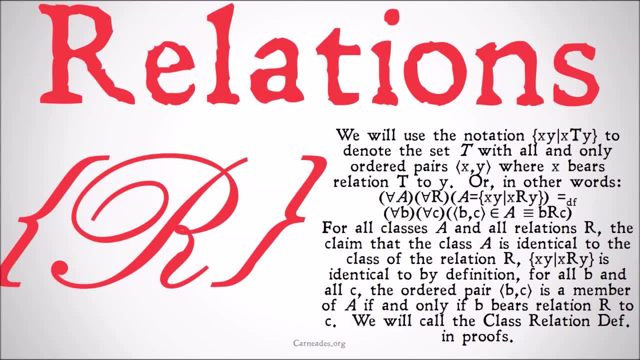 a is materially equivalent to b bears relation r to c. We're going to call this class relation definition in proofs Now, broadly, in set theory. you are only going to be instantiating these things into classes and sets, but we are giving a very broad definition here, one to help understand it, but also so that we